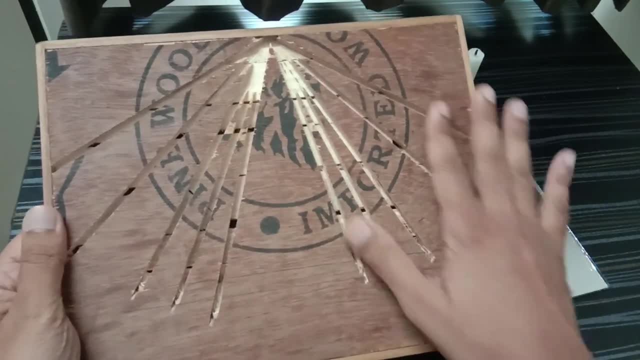 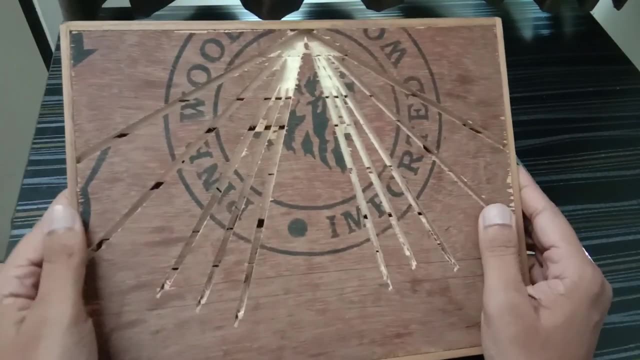 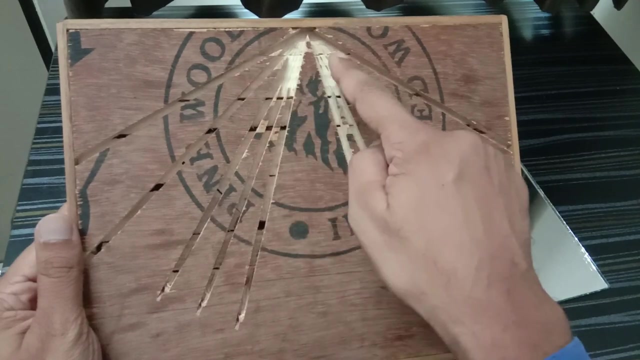 most important part of our experiment. I asked my carpenter to make some grooves on a piece of wood- This is a simple plywood of 18 mm thickness- and I had drawn two lines, this one and this one having angle 120 degrees, and I gave it to my carpenter and this is. 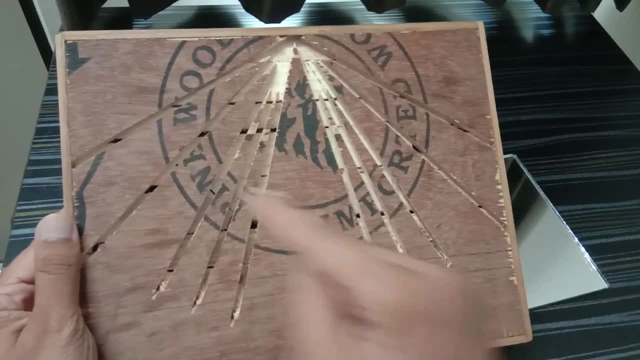 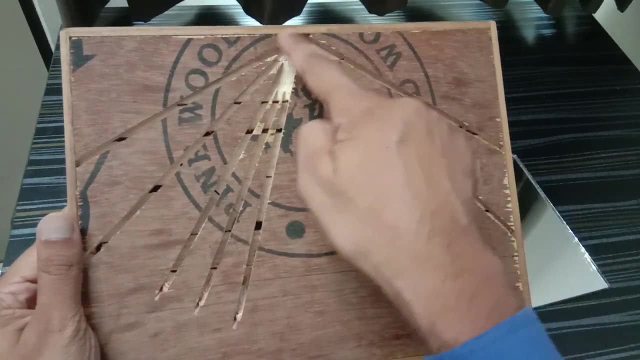 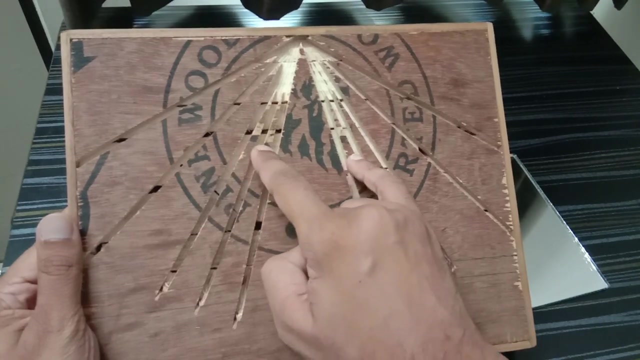 4 mm in thickness, because the plane mirrors are approximately 4 mm thick, So he had made the carvings of 4 mm thickness. Now, this one and this one, these two lines are at 120 angle. these two lines are at 90 degree. these two lines are at 60 degree, these two at 45. 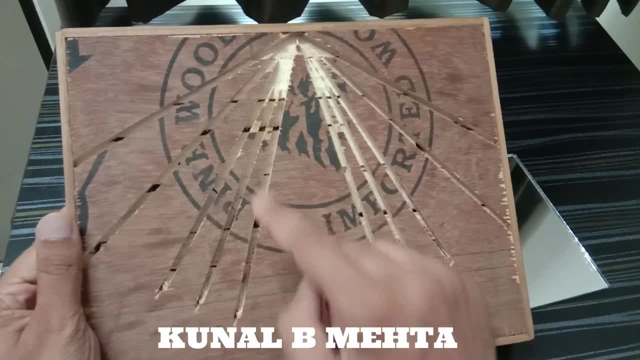 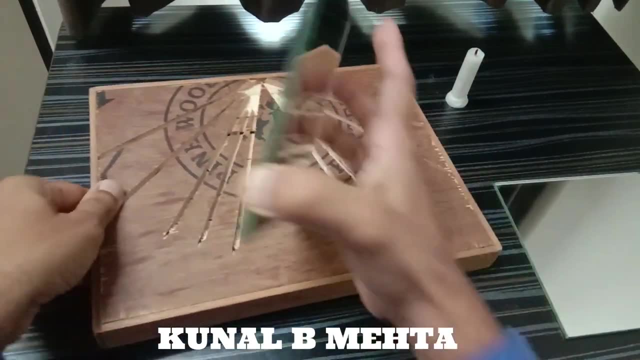 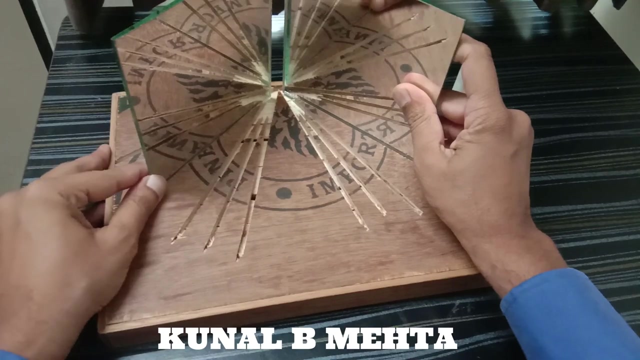 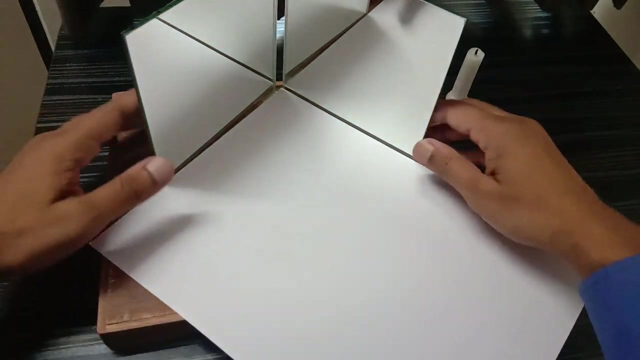 and the last one. last these two lines at 30 degree, correct? So I am going to arrange the mirrors at 90 degrees like this. Also, I am going to put an A4 size of paper over here. Now I must ensure that both the 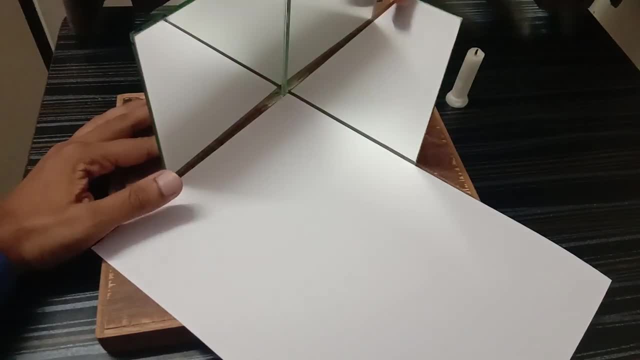 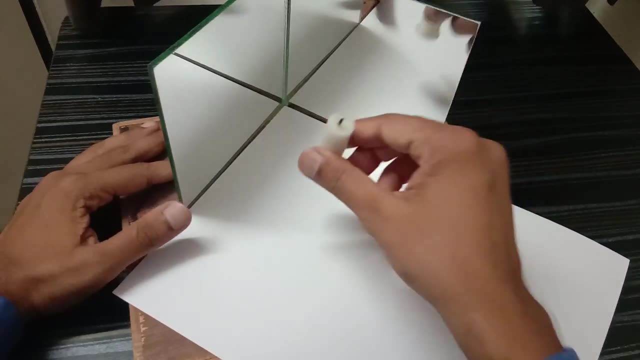 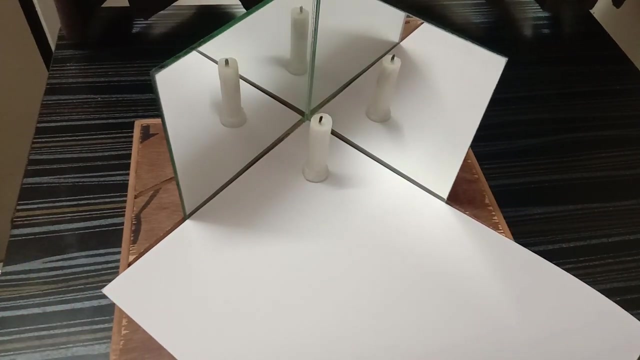 mirrors are joined together properly, Okay, done. Now what are we actually doing in this experiment is this is our object, and I am choosing to keep the object over here. Now, there are two positions in which you can keep the object. 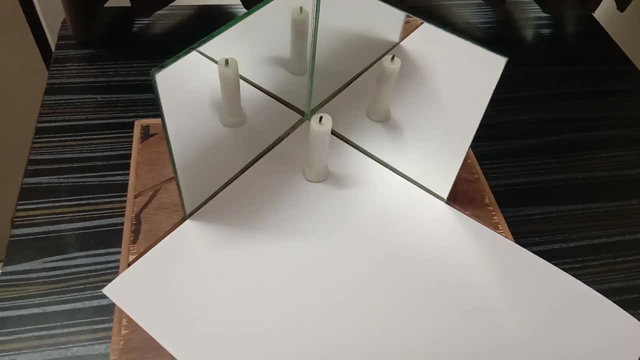 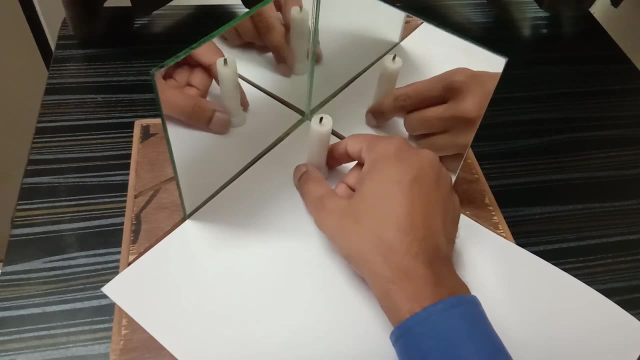 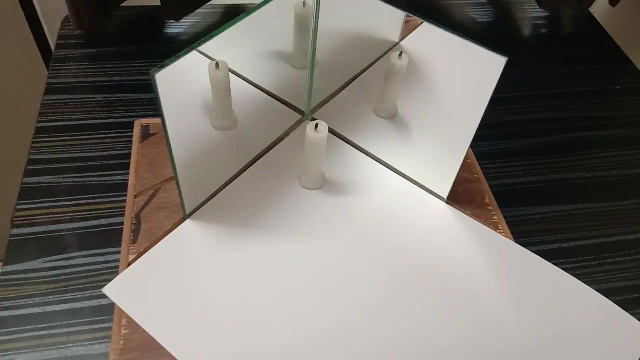 One is on the angle bisector of the mirror. that is called the symmetric arrangement of the object from both the mirrors. So you can do that. So here, if I keep an object on the angle bisector, that means from this mirror. this angle is 45 degree, and from this. 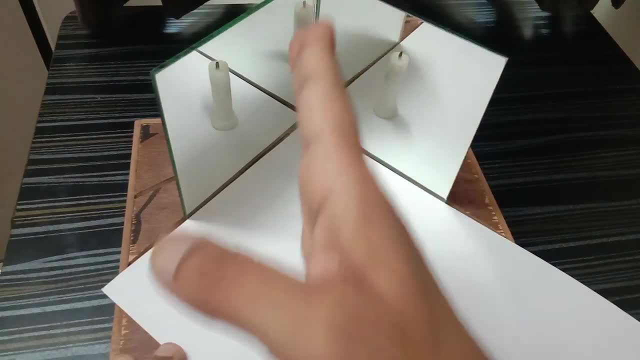 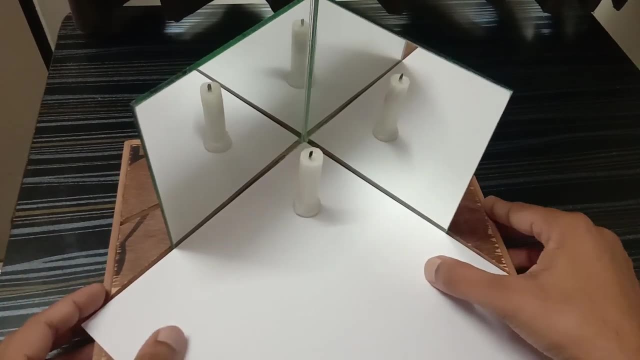 angle. also, the angle is 45 degree, So exactly on the angle bisector line, symmetrically, I am putting the object. Now let me say one thing: What is going to happen over here is now, since there are two mirrors, I am going to 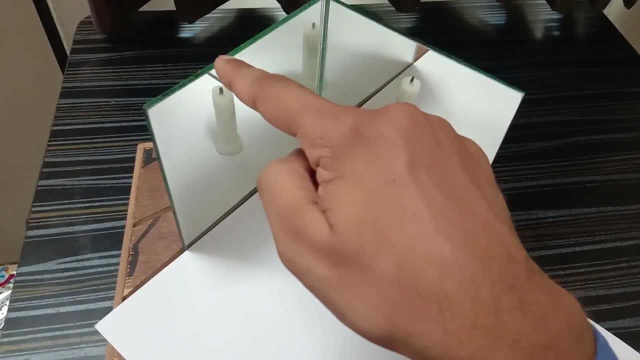 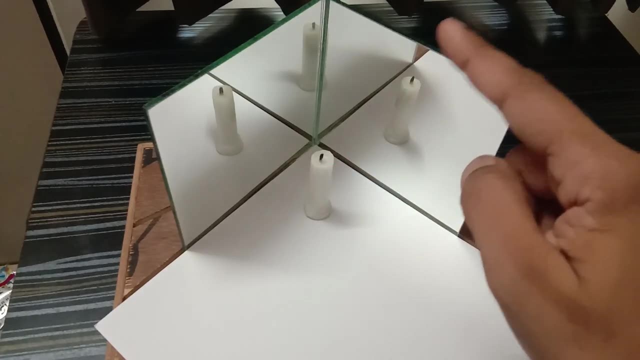 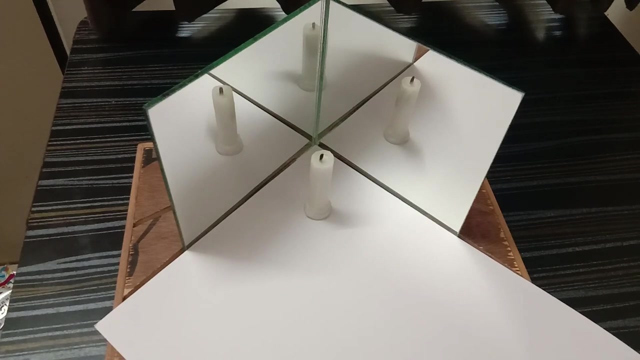 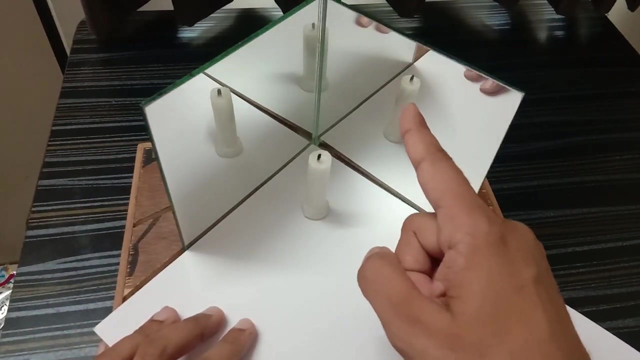 call this as mirror M1, this as mirror M2, right, This is the first image of this candle in mirror M1 and this is the second image, and this is also the first image of this candle in mirror M2.. These two are called the primary images. Now this primary image will behave as the 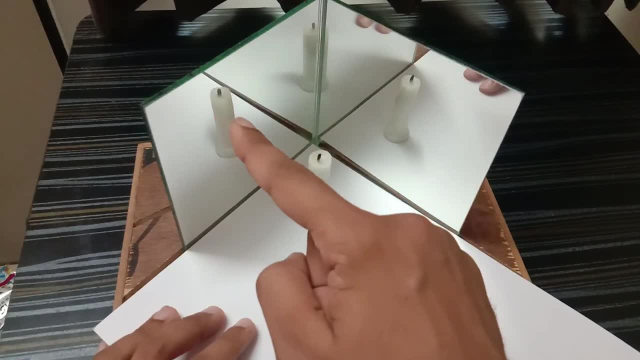 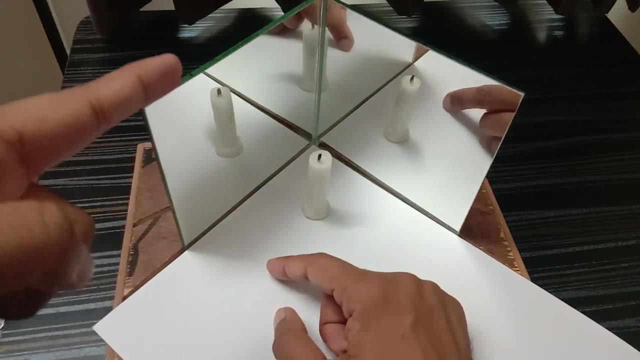 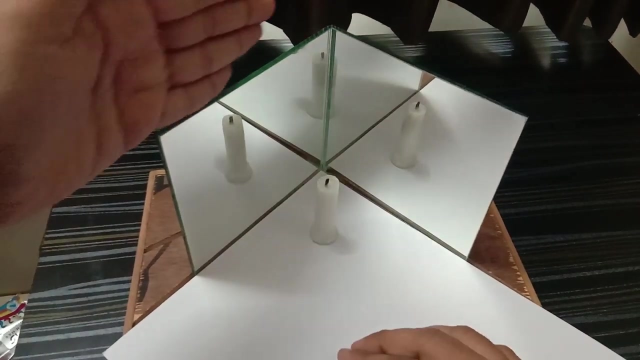 object for the image of this mirror. guys See, this image is visible over there, The image of this mirror is visible over there and we can also consider that we can extend this mirror behind. So this is our extended mirror behind. We can extend the mirror behind. 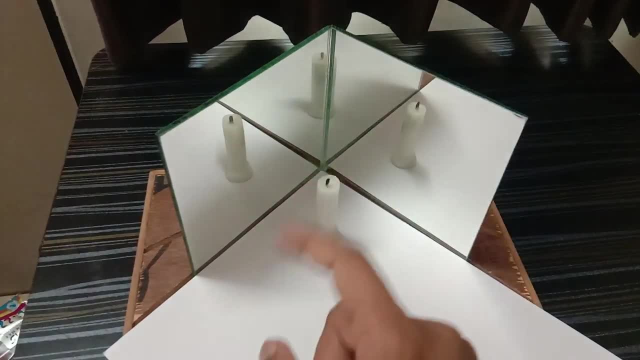 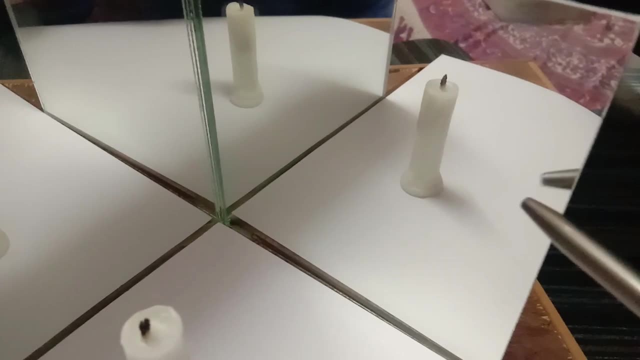 So this image will behave as an object. For that we have to keep the object. So here we have that extended mirror and its image will be formed on the other side. Let me show you that, So that is very well visible, that now this image will behave as the object for that mirror. 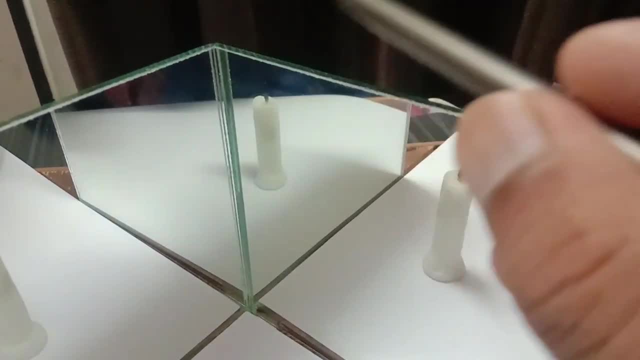 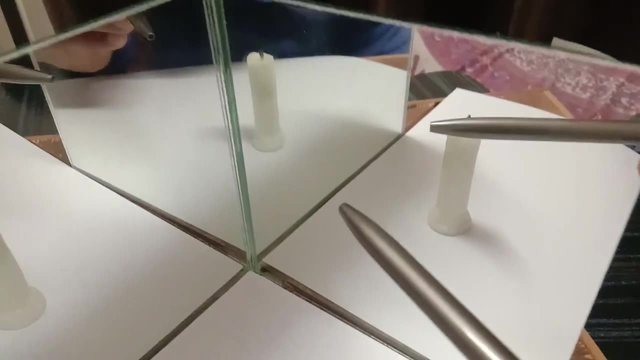 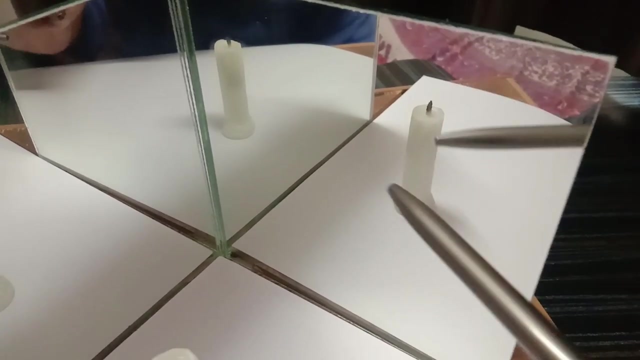 which is the extended. We can consider this mirror to be extended behind, or that is the image of this mirror in this mirror, or, simply, you can consider this as the extended mirror and that that is the secondary image of this primary image, because this is behaving as 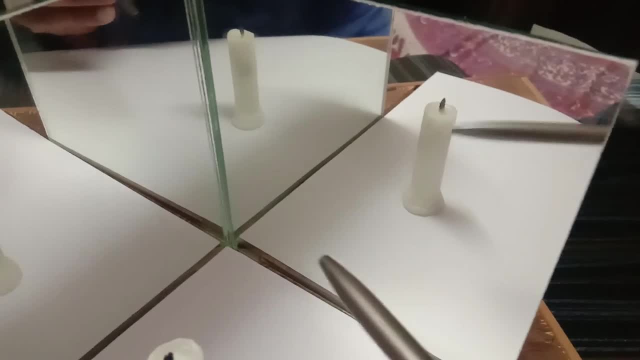 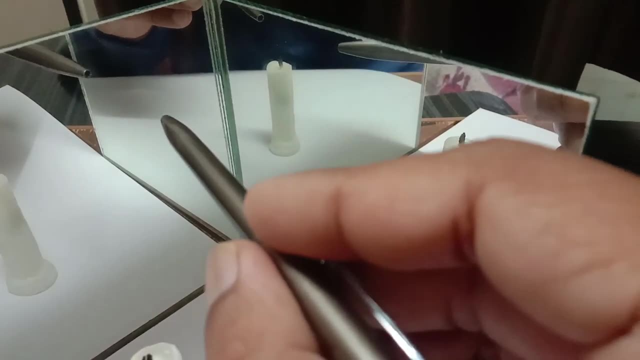 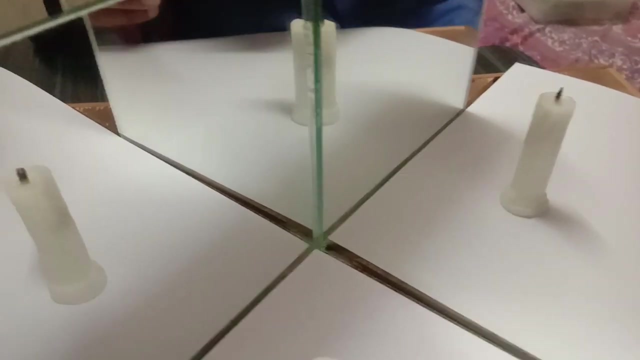 the object for that mirror. Now, this secondary image cannot behave as the object, because you can see that this is the reflecting part of the mirror and this image is formed behind the mirror. So you have to stop there And the total number of images that you are seeing. 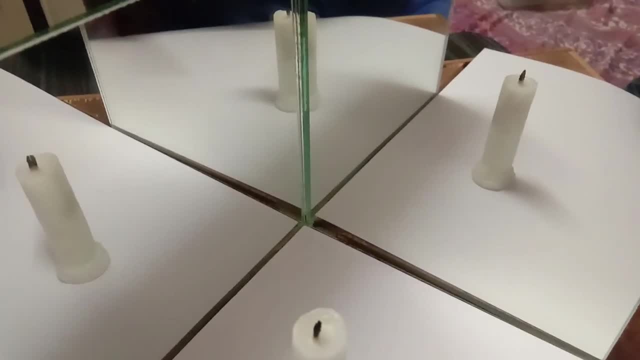 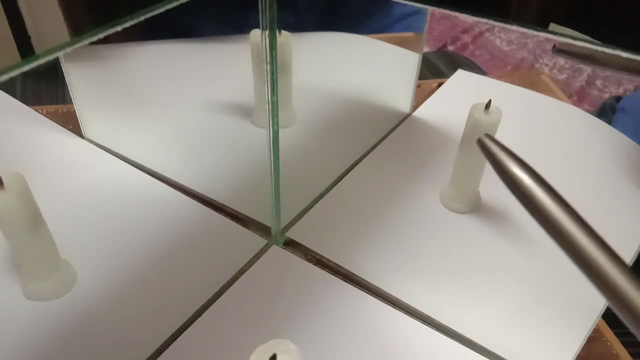 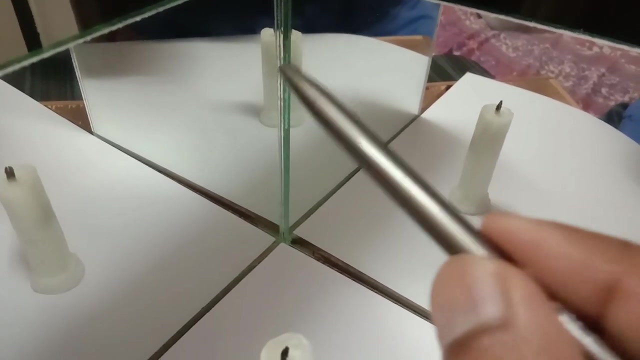 in this case is three. Now, guys, sometimes what happens is there are four images, but the last two images are falling on one another, like in this particular case. The image of this is here and the image of this is coinciding on that one, So we are considering that image. 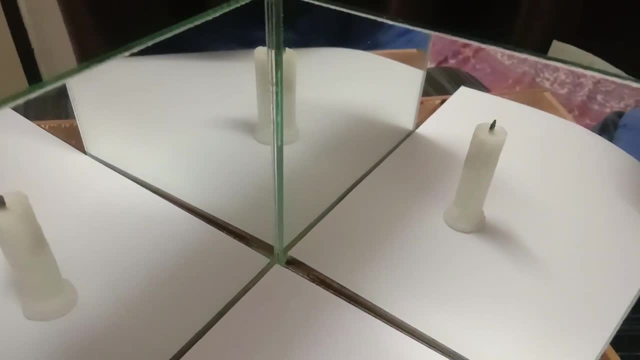 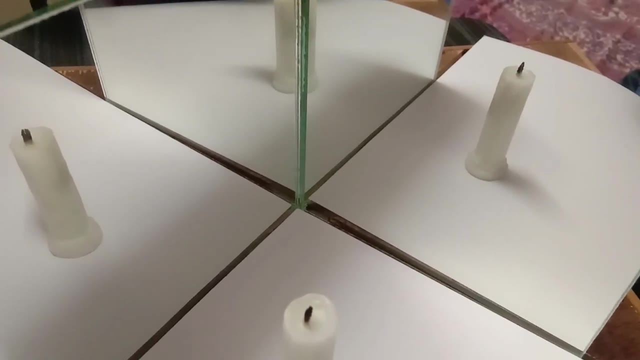 as the one image. Actually, there are two images, but they both are coinciding on one another. So hopefully, guys, I have told you what is the theory part, And now let's start the experiment by keeping the angle between the mirrors as 120 degrees. 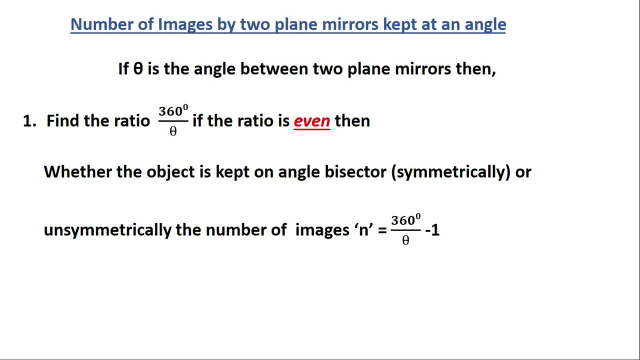 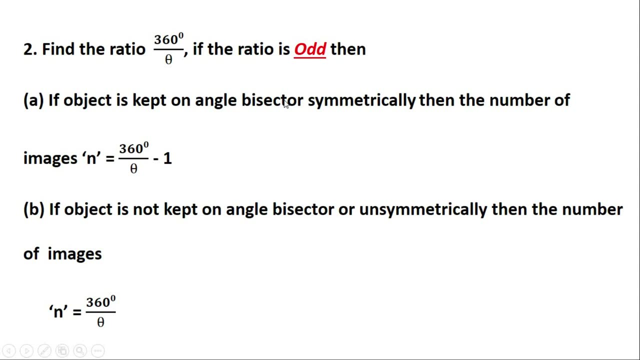 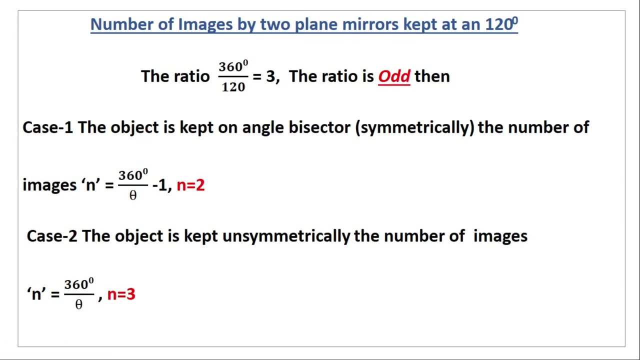 All right. So we are going to do the experiment for this first image. So we are going to start with the two side mirrors. We are going to try to set them to be on this side and that side too. All right, 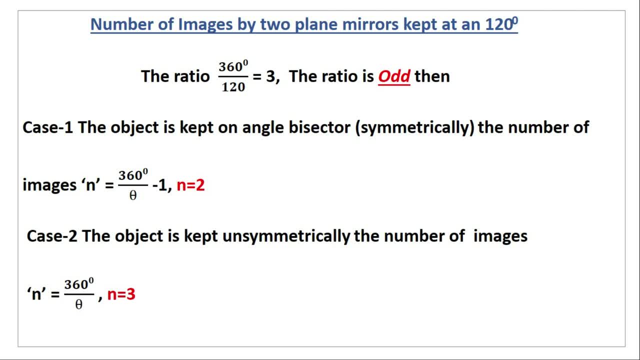 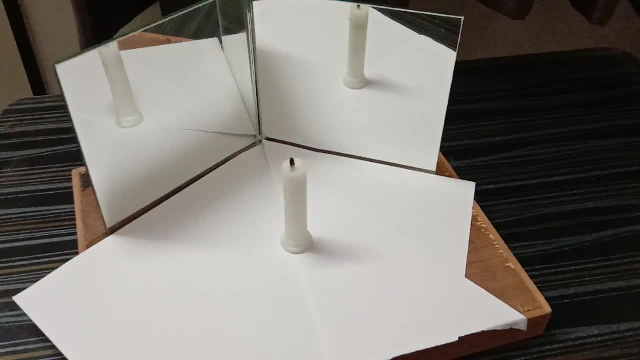 So this is the second image, All right, All right. so, guys, now the setup is ready and the angle between both the mirrors is 120 degrees. this angle is 120 degrees and this is the candle, which is exactly at 60 degree from both the mirrors. so 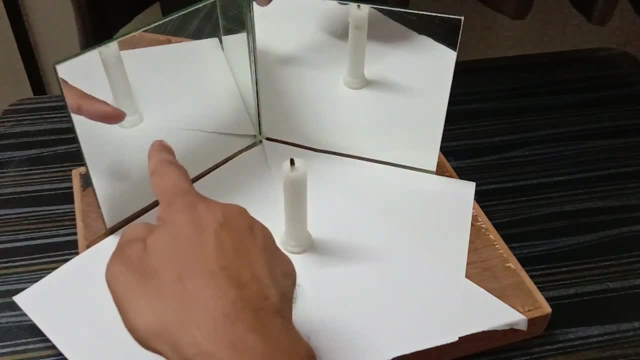 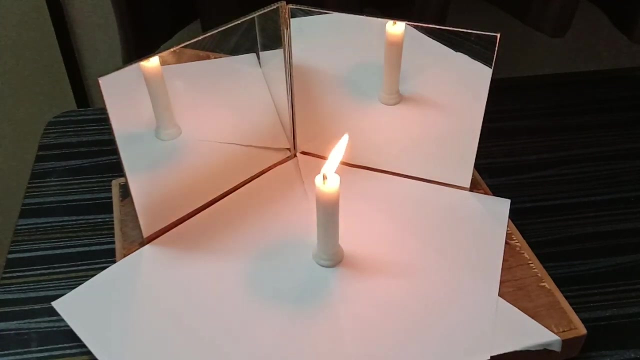 it is on the symmetrical distance from both the mirrors: from here also 60 degree, from here also 60 degree. now the formula says something like this: you can just see on the screen. so here, from a distance, we are able to see two images. let me show you by bringing the. 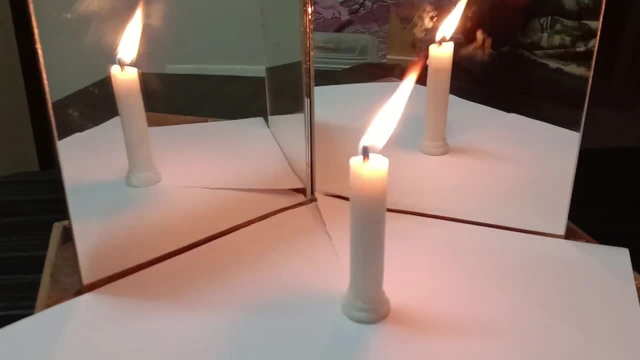 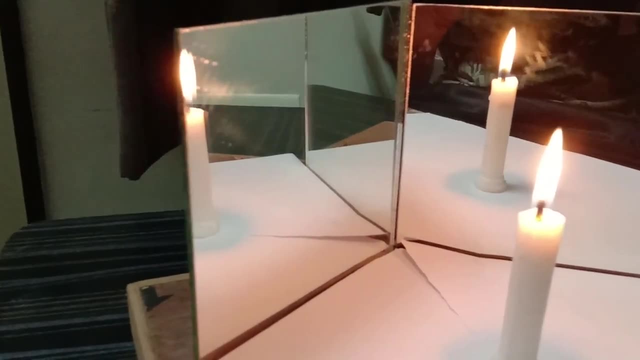 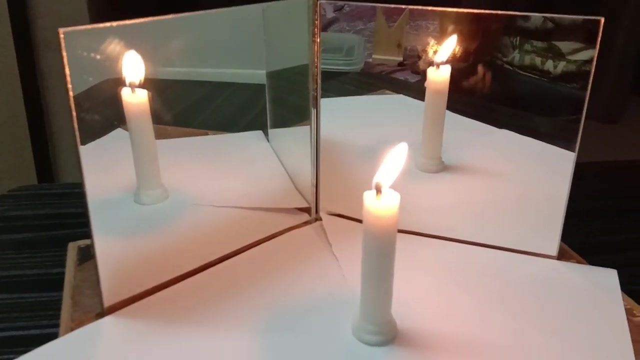 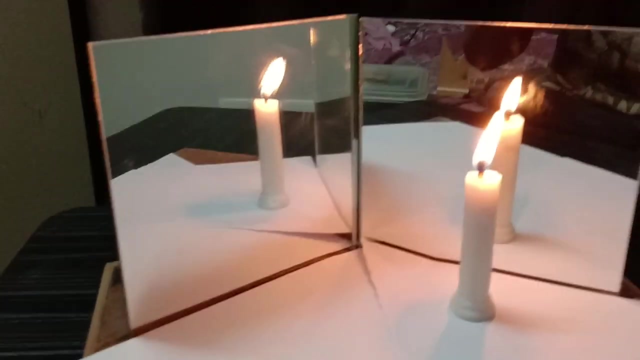 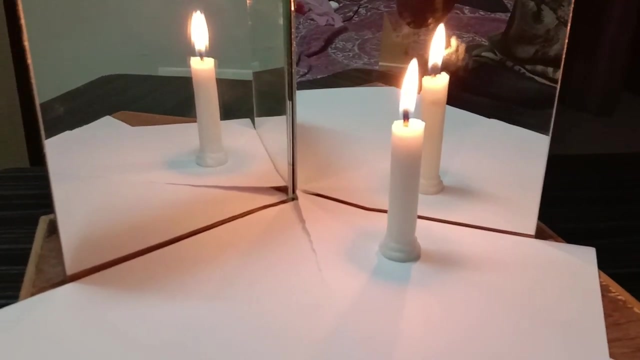 camera more nearer. so, guys, there are two images which are formed and you, if I've move around a bit, there is no third image which is seen. but if I displace this candle somewhere over here and if I keep it at some asymmetric distance from both the mirrors, the number of images tend to change, guys. so 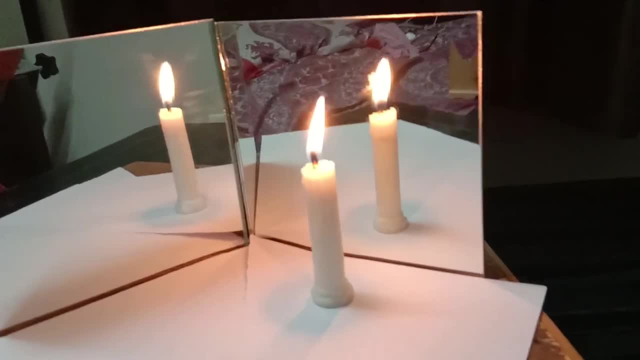 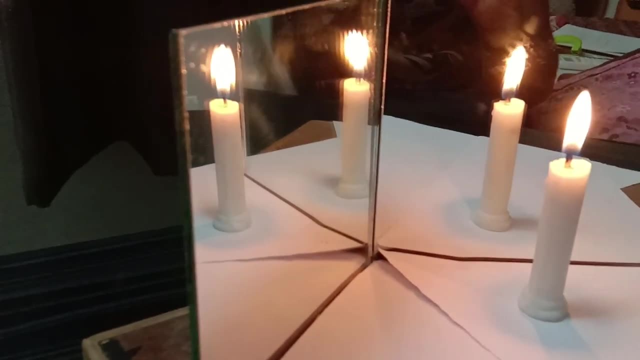 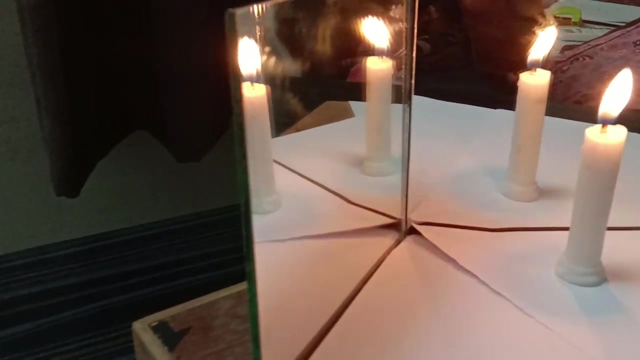 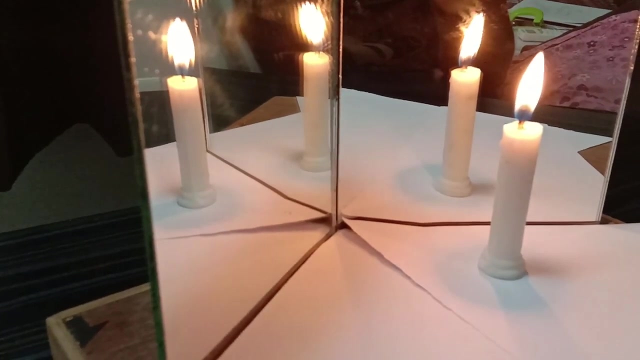 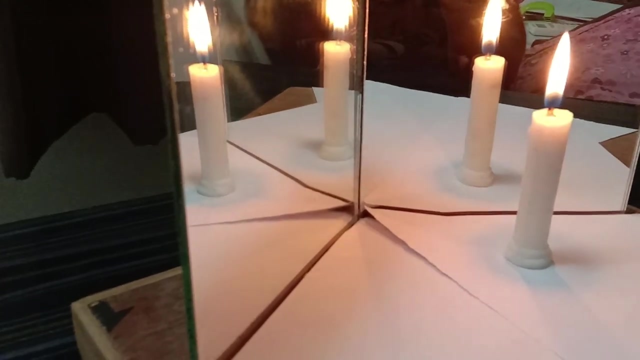 this is the first image, that is the second image and if you you there, you see there is a third image. guys, so total, there are three images which are obtained when you keep this candle or the object at different distances- that means asymmetrical angles or distances- you will find three images. 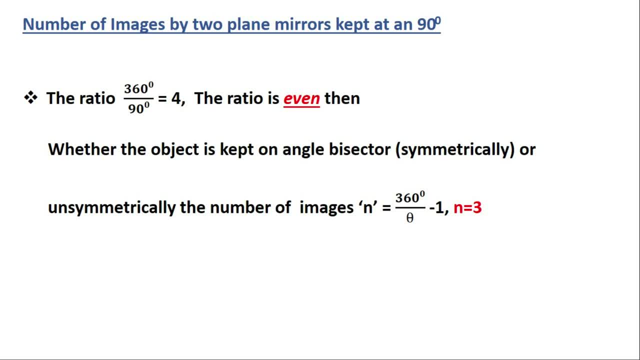 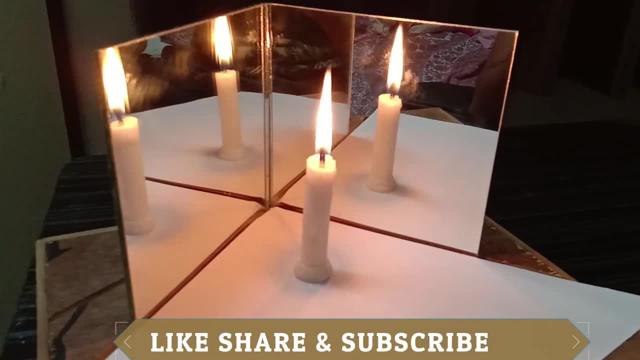 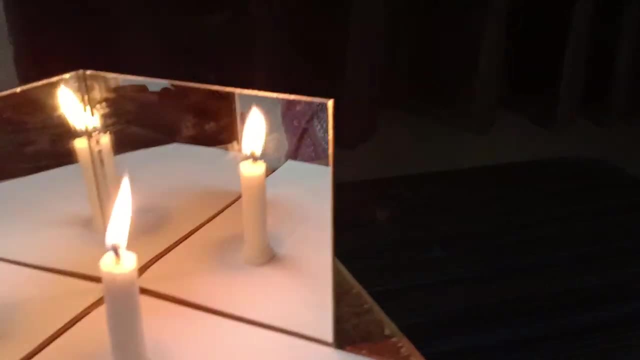 and that increases this value thanks to its vertical position, as you see here, and this way, this is really nice, delicious. even if you go here the first, I will move the camera a little bit here. this is because it raises height, so I need at least few moments driving. 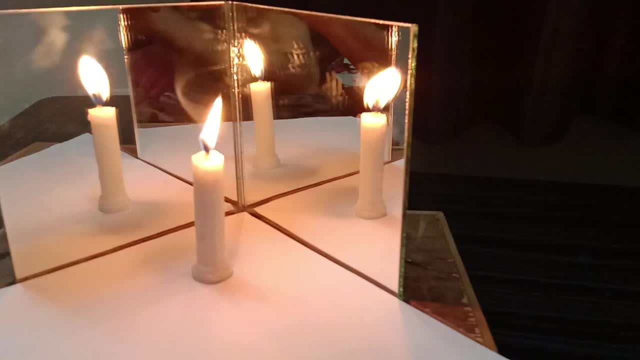 with the direction sight in pointiness not so much a little, but you know you may not. by using another indicator at any time you can set the same time. i make sure i do this at any time so i can sift through the connective card and i set a cheque and affect it and how it will open up its, thereby save you your idea right now. 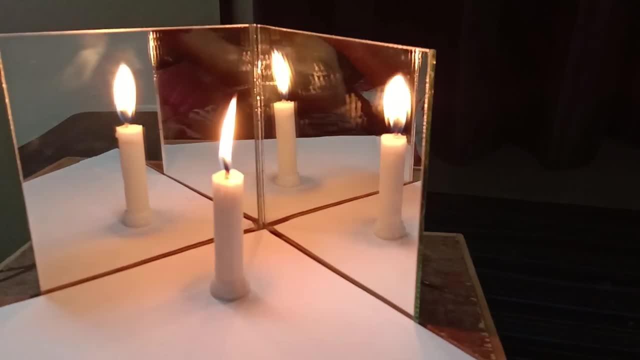 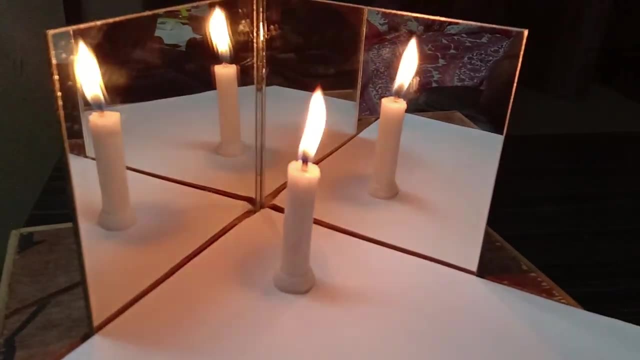 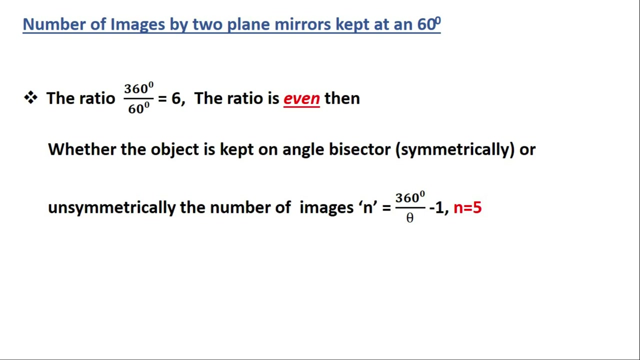 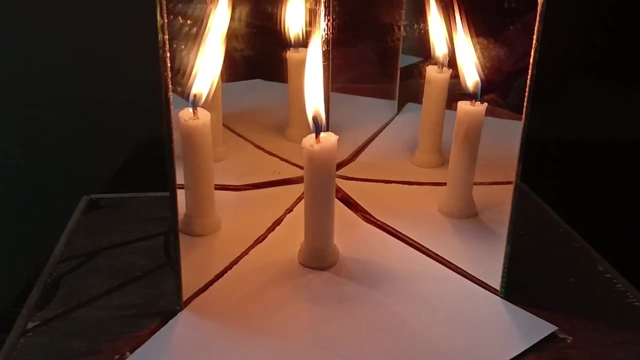 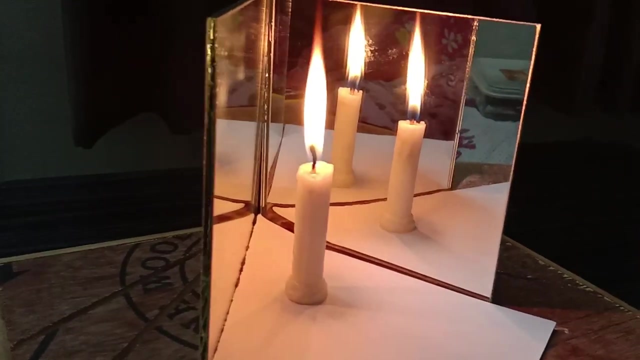 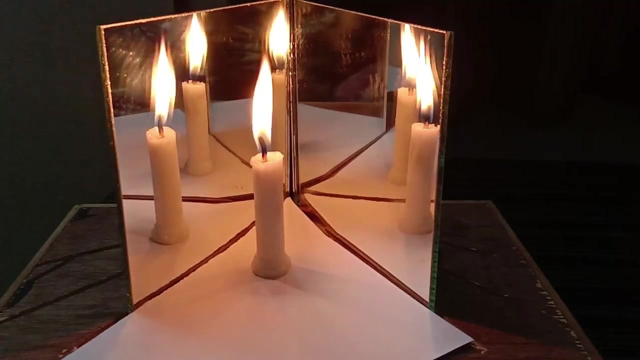 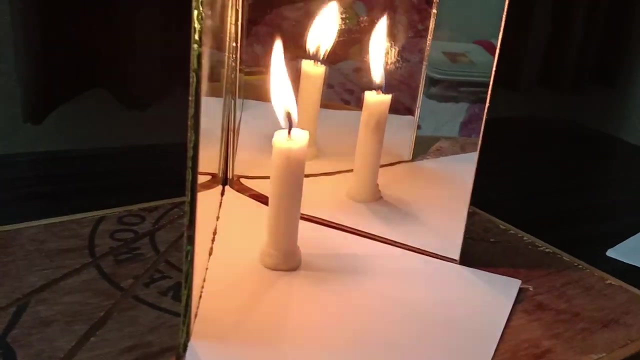 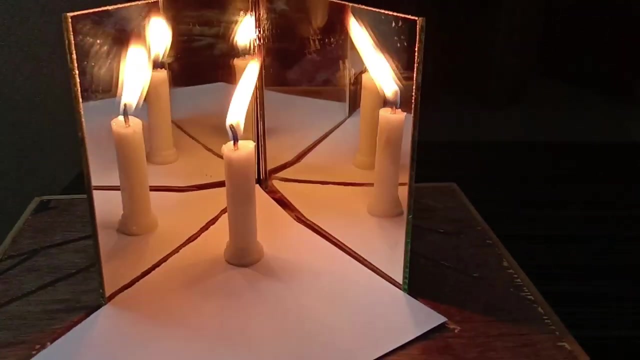 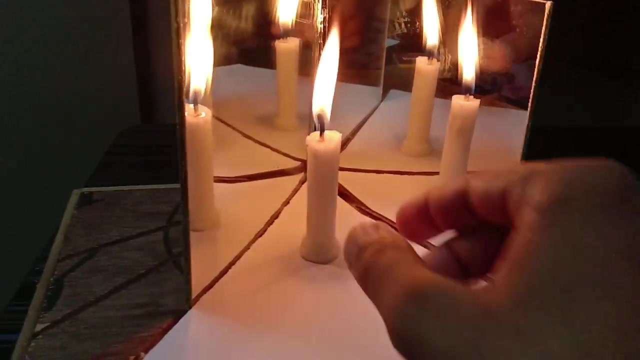 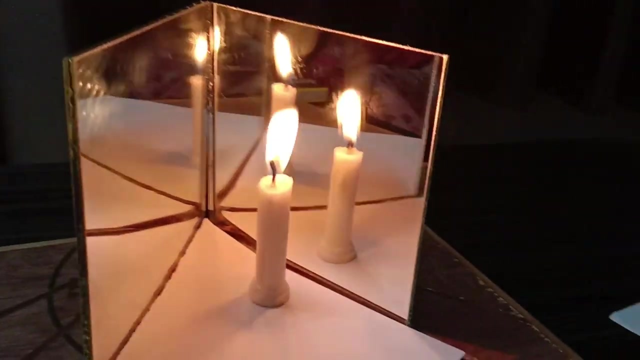 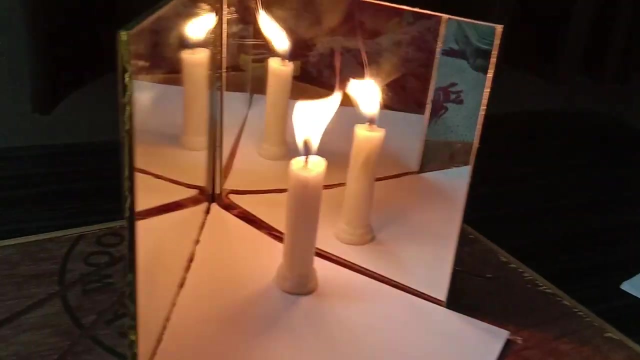 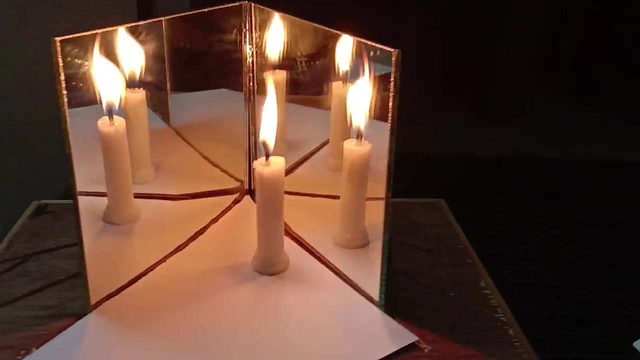 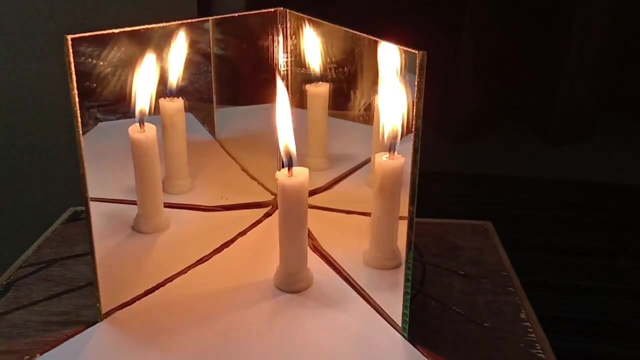 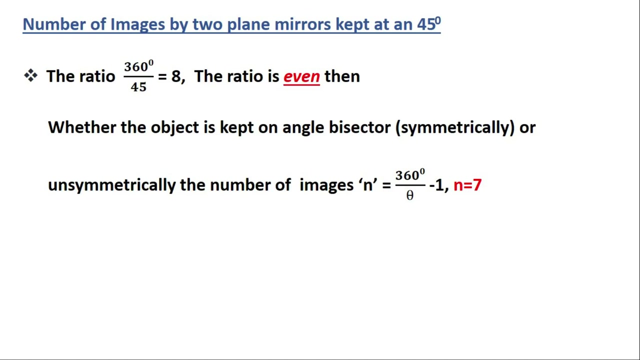 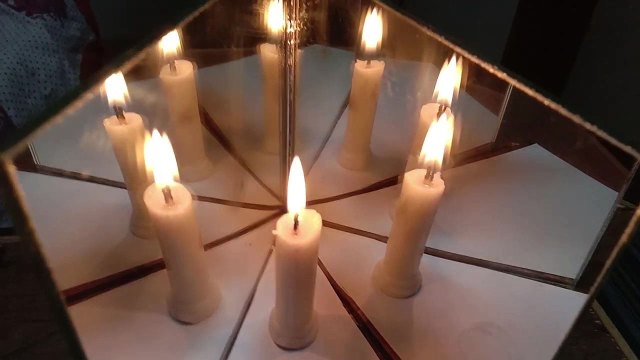 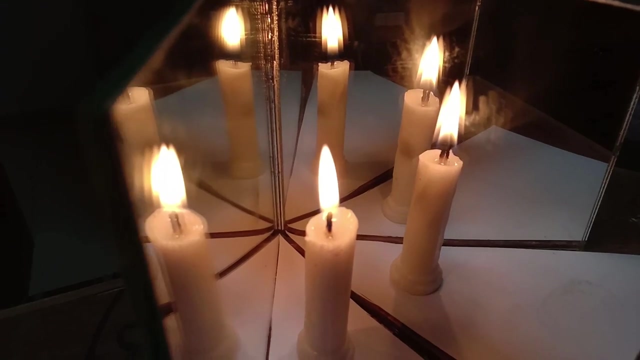 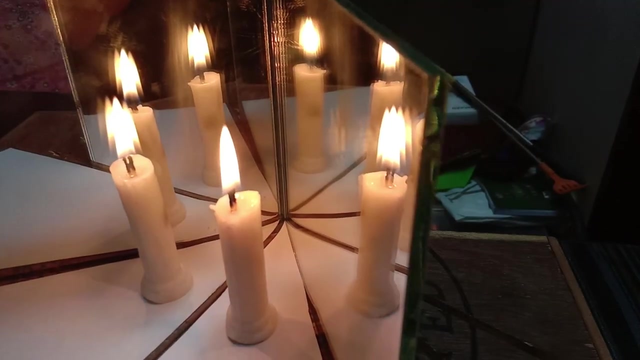 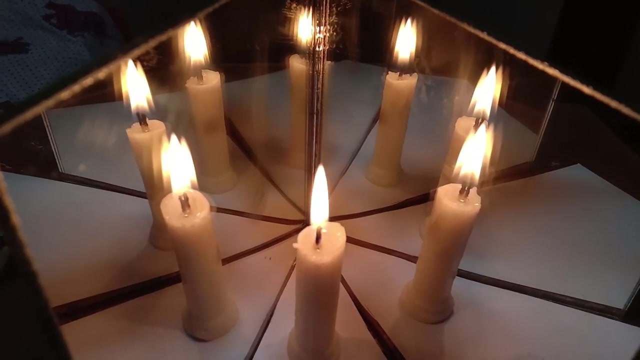 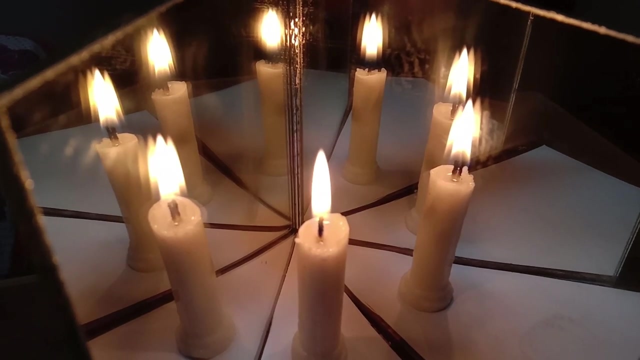 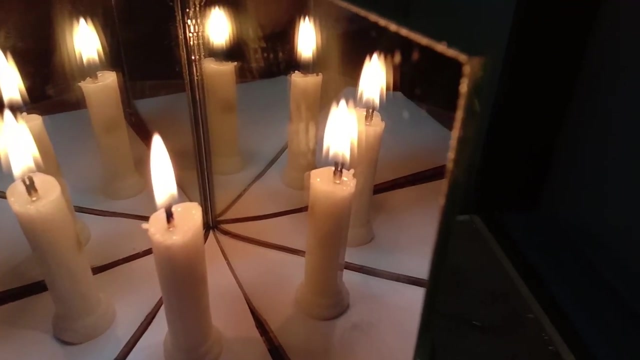 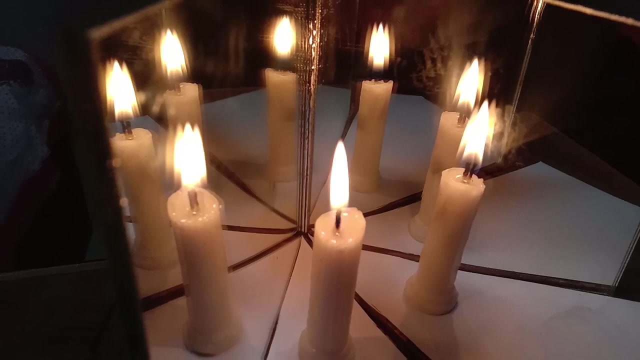 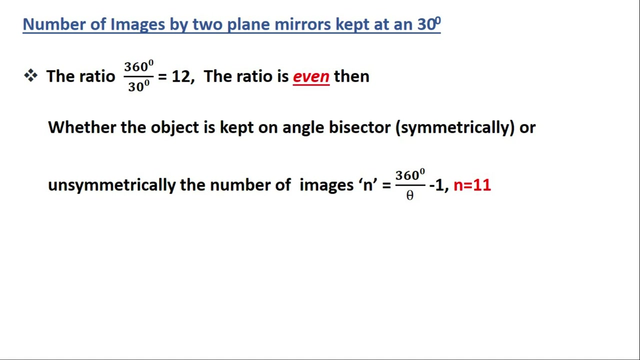 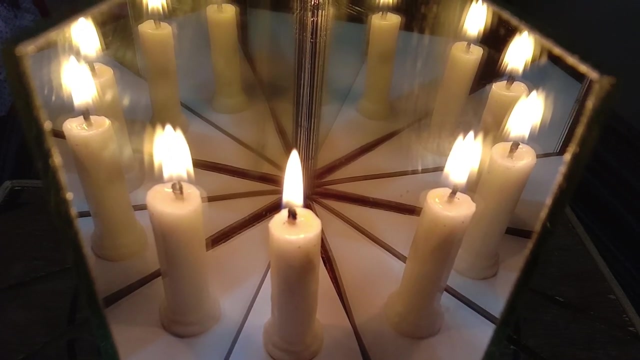 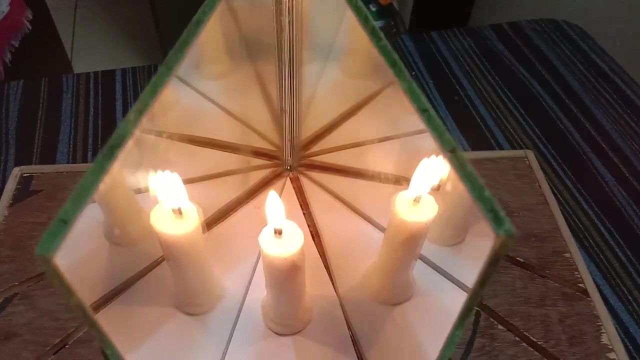 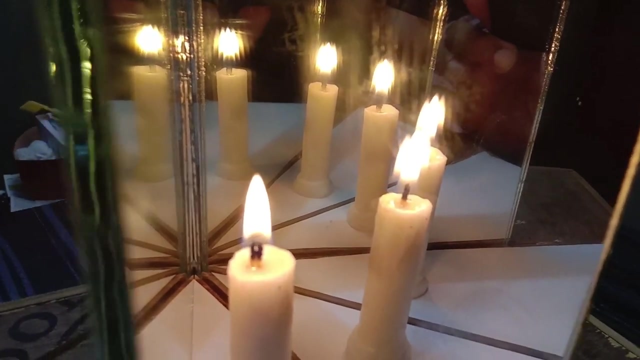 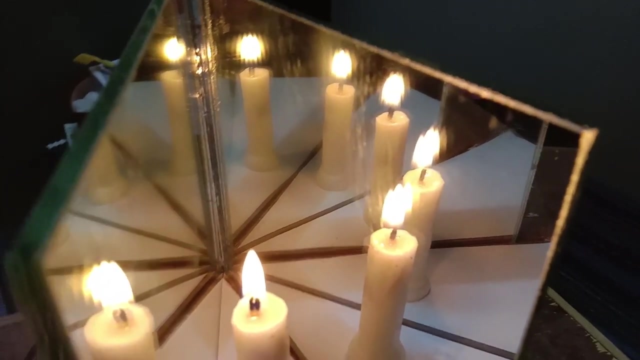 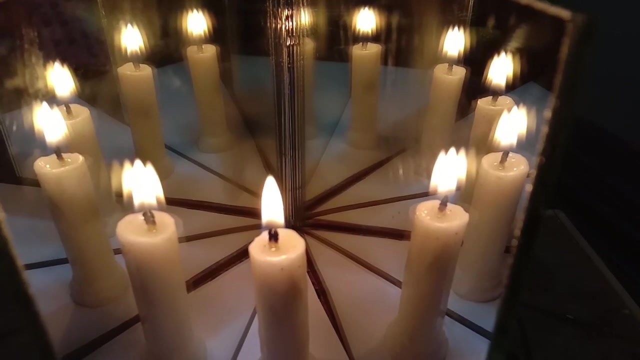 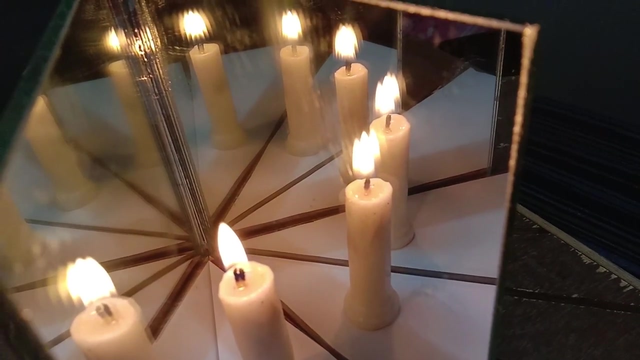 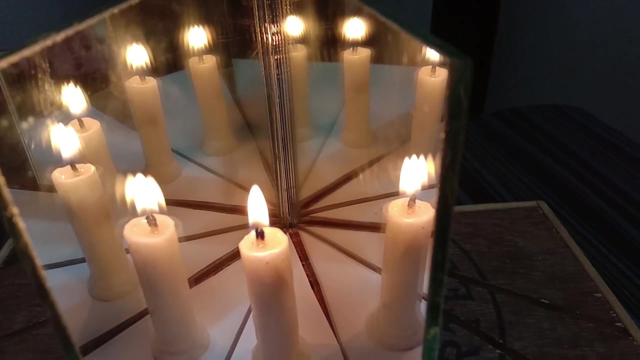